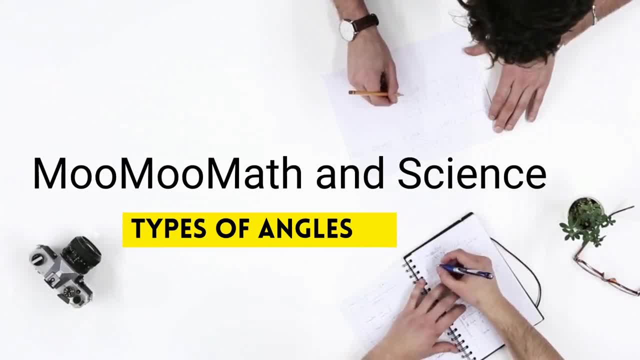 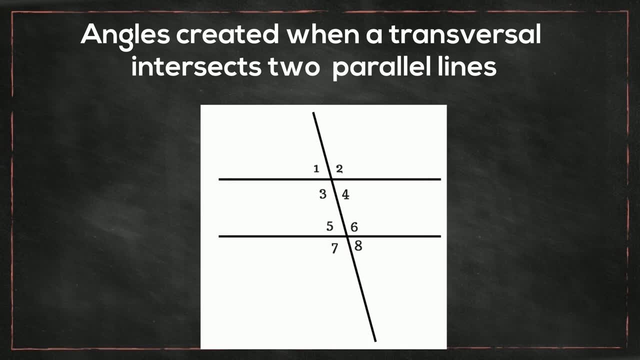 Welcome to MooMooMath and Science. In this video I'd like to look at angles created when a transversal intersects two parallel lines. We'll first look at the angles and angle pairs and their relationships, and then we'll work. a very short problem. 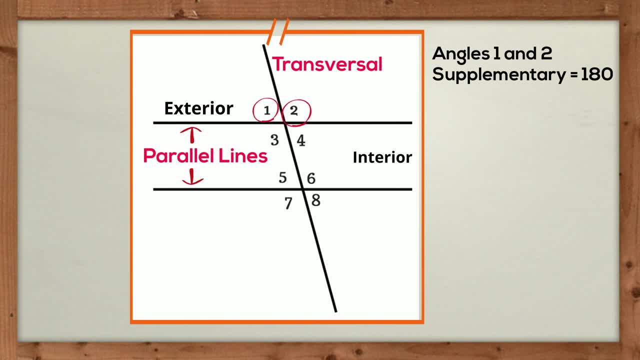 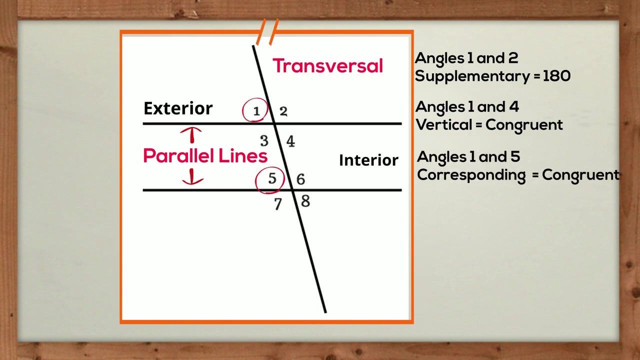 Okay, first angles one and two. they are next to each other, so these angles are supplementary, so their angle measure added together equal 180 degrees. Angles one and four are called vertical angles and their angle measure is congruent or equal. Angles one and five are called corresponding. 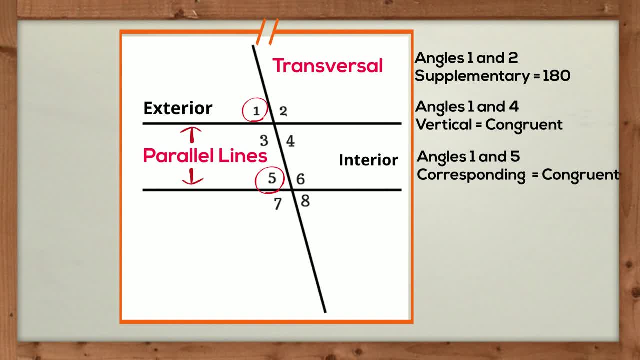 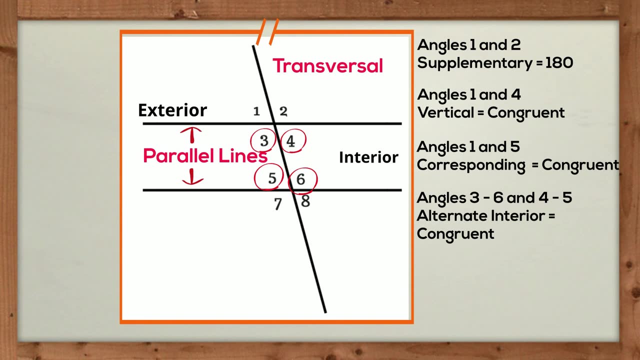 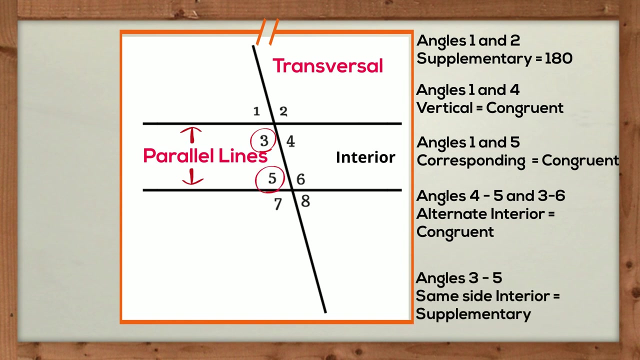 angles and they also have congruent angle measures. If you look at angles three and six and four and five, these are called alternate interior angles and they also have congruent angle measure. Angles three and five are same side interior and they are supplementary. 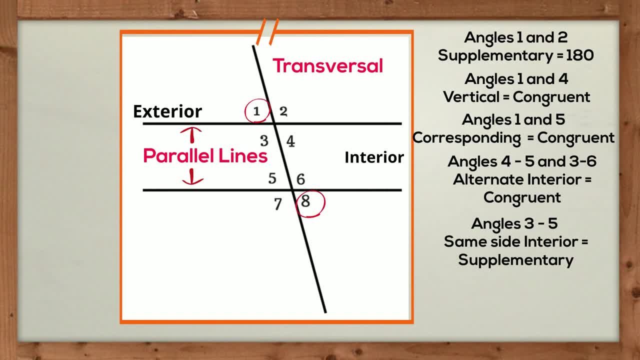 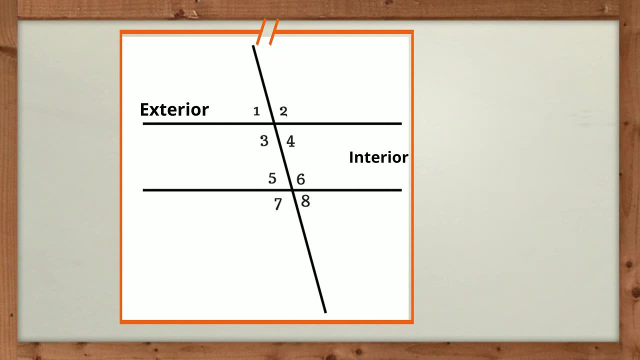 And finally, if you look at one and eight, these are called alternate exterior angles and they also are congruent. Now, I didn't name every single angle here, but examples, and so you can locate different ones. Okay, let's look at a quick question. Let's find angles one, two, three and four. 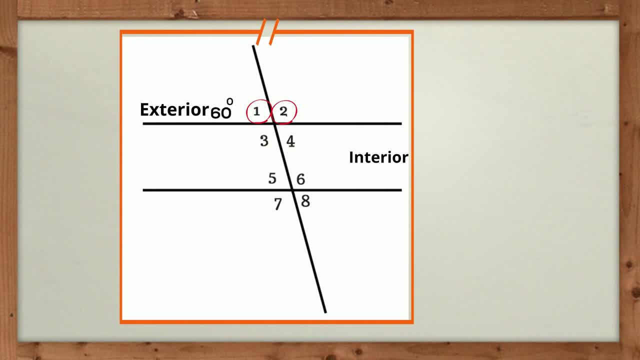 if you know that the angle measure of one is sixty degrees. Well, since one and two are supplementary, I take 180 minus sixty, and that equals 120.. Angles two and three are vertical, so angle three: they are congruent. so angle three are congruent. 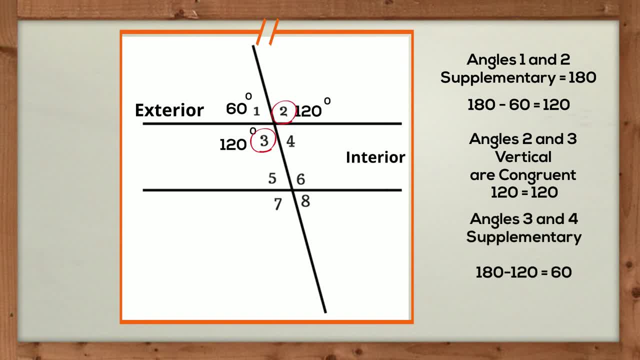 Angle 3 will be 120, and then angles 3 and 4 are supplementary. so 180 minus 120 equals 60. Now how about if angle 1 again is 60 degrees? what is the angle measure of 8?? Well, they are alternate exterior and they are congruent, so that would be 60 degrees.